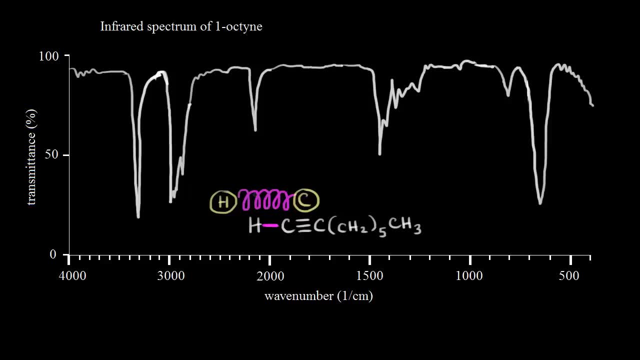 on the other side, And so the stretching vibration of the bond is like the oscillation of the spring. So if you had a spring and you had two masses on either end of the spring, if you put some energy in you can stretch that spring. 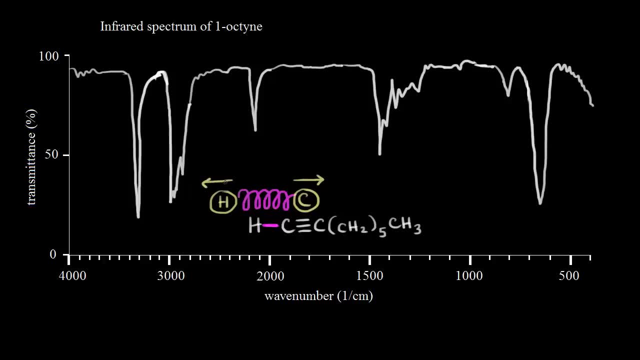 So you could. you could pull the carbon this way, you could pull the hydrogen that way, So that's like the stretching of this bond here, And we know that springs also contract, So then the spring could pull back in this direction And you get an. 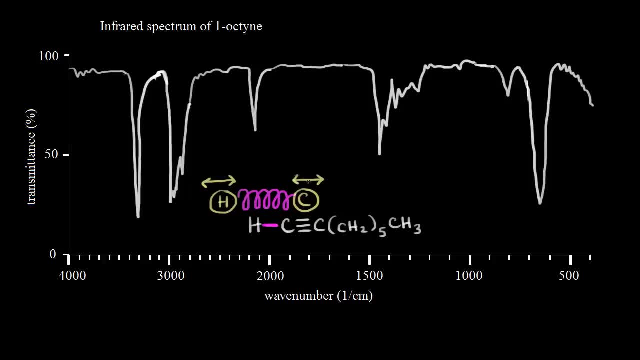 oscillation of the spring, which is once again how we model the stretching vibration of a bond. So let's look at the IR spectrum for this molecule. So we're talking about one octane here And, if you shine, a range of infrared frequencies. 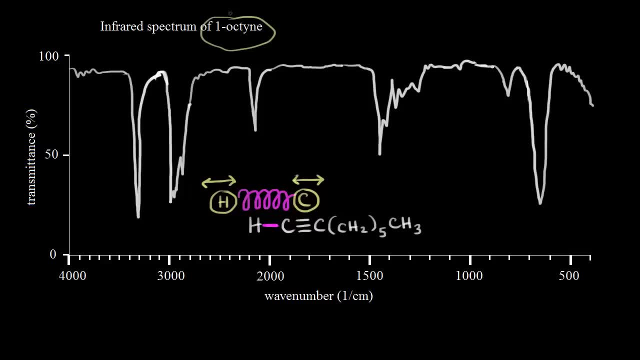 through a sample of this compound. some of the frequencies are absorbed by the compound And you can tell which frequencies are absorbed by looking at your infrared spectrum here. So for right now, let's think about these numbers like 3,000 or 4,000.. Let's think about those as representing frequencies. 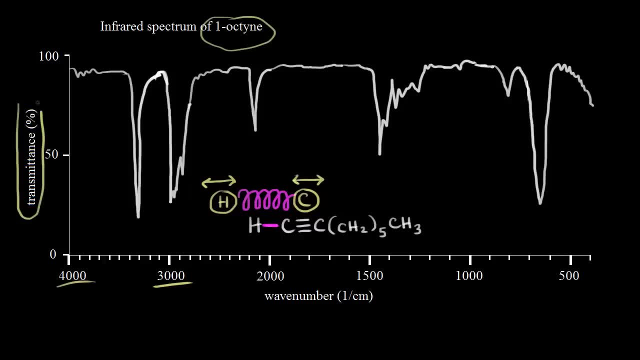 of light, And so over here we have percent transmittance, And so if you had a 100% transmittance, let me go ahead and draw a line up here. So 100% transmittance. So let's say we're talking about this frequency of light. 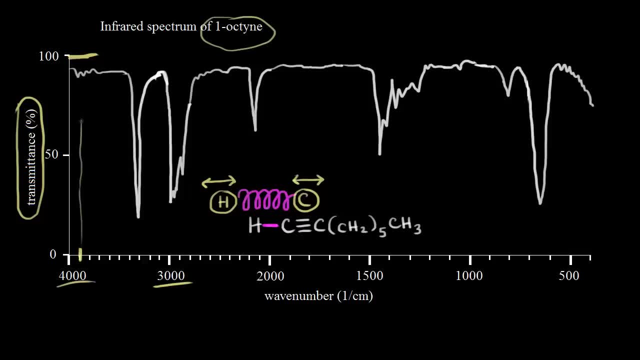 So I look at this frequency of light, I go up to here And I can see I have 100% transmittance. 100% transmittance means all of that light was transmitted through your sample. If all the light went through your sample. 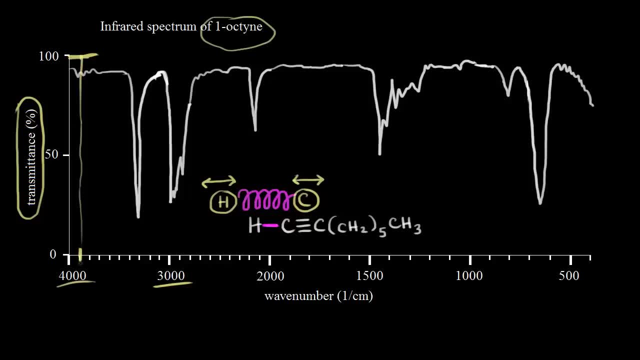 nothing was absorbed And so this particular frequency was not absorbed by your compound. So if you're talking about less than a 100% transmittance, let's say for this frequency right here. so for this frequency we have this signal here appearing at this frequency we don't have a 100% transmittance. So that means that you've got a 100% transmittance. 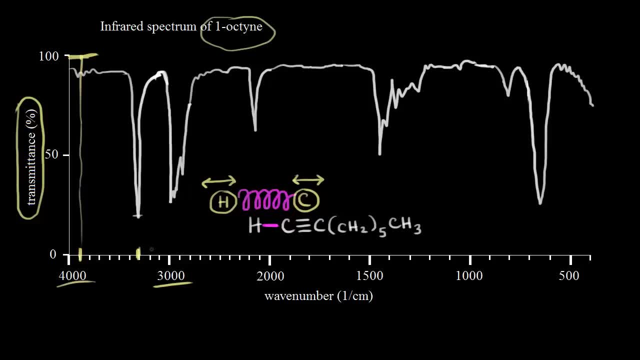 is not all of the light went through the compound. Some of it was absorbed, all right, So some of that. so this specific frequency was absorbed by the molecule and that energy can cause a bond to stretch and we get a stretching vibration. 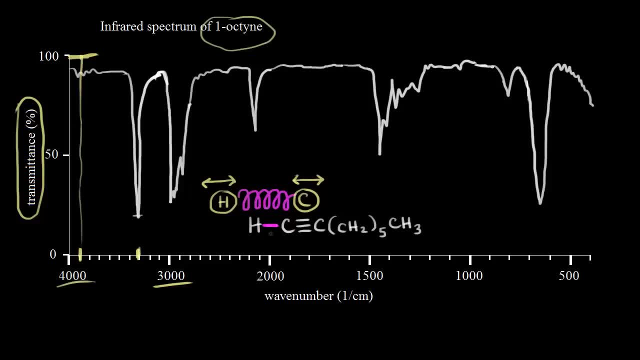 And actually this signal corresponds to the bond that we've been talking about. So this signal indicates the stretching of this bond right here. All right, let's think about wave number next. We just talked about percent transmittance. Let's think about wave number. 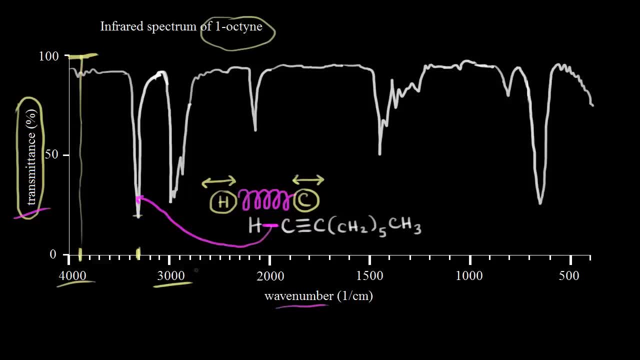 So I've been calling all these things frequencies, different frequencies of light, and let's see how wave number relates to the frequency of light and also the wavelength of light. So the definition of wave number, so a wave number. here's the symbol for wave number. 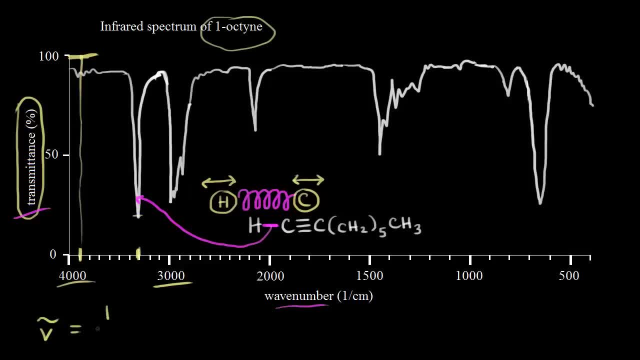 the definition of wave number is it's equal to one over the wavelength in centimeters. All right, so if we had a wavelength of light of .002 centimeters, so let's go ahead and plug that in, so a wavelength of light of .002 centimeters. 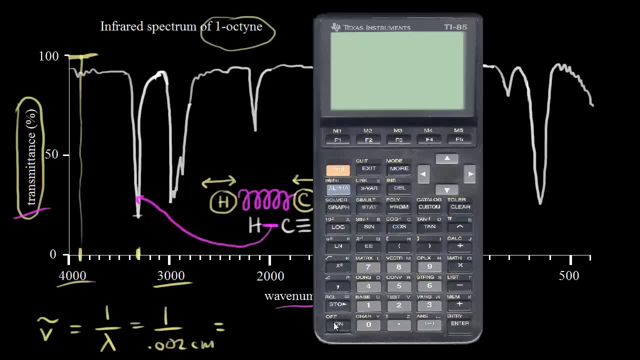 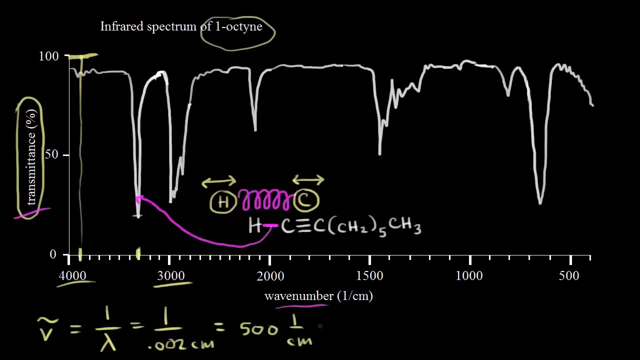 what would be the wave number. So let's get out the calculator here and let's do that math. One divided by .002 is equal to 500.. All right, so that's equal to 500.. Your units would be one over centimeters. 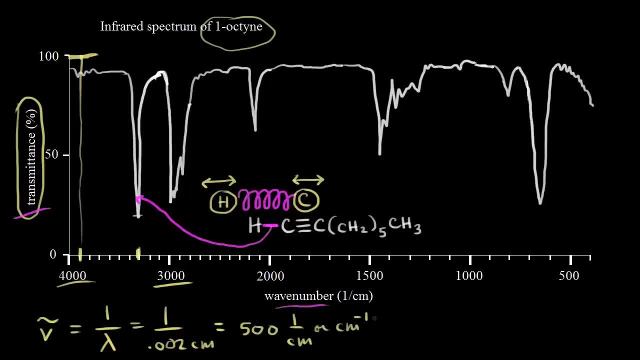 or you could write that meaning the same thing. So that's the wave number. that's the wave number. So if we go over here, right, a wave number of 500, you could think about this corresponding to a particular wavelength of light. 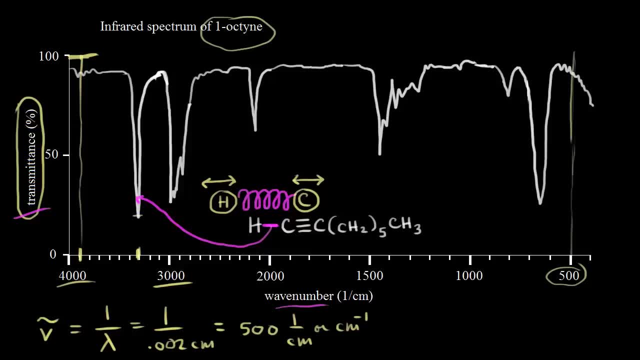 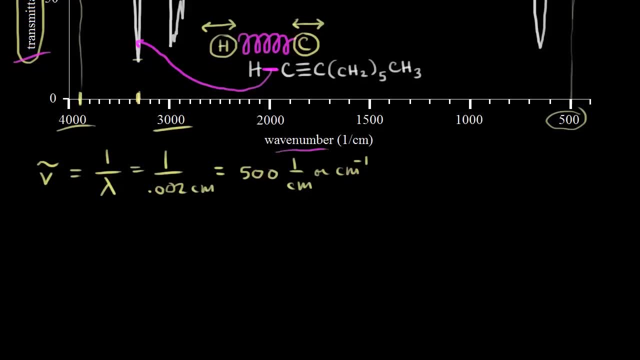 and of course this also relates to frequency, because we know that wavelength and frequency are related to each other. so let's get some more room down here. and we know that the wavelength times, the frequency, wavelength times, the frequency, so lambda times nu. 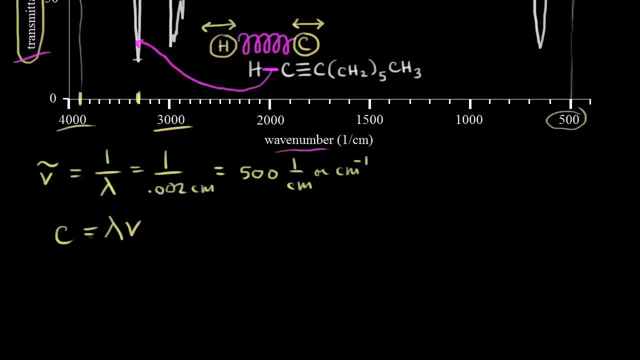 is equal to the speed of light, That's equal to c. All right, so if I wanted to solve for the frequency, so solve for nu. the frequency is equal to the speed of light divided by lambda, divided by the wavelength, And that's the same thing as one over lambda. 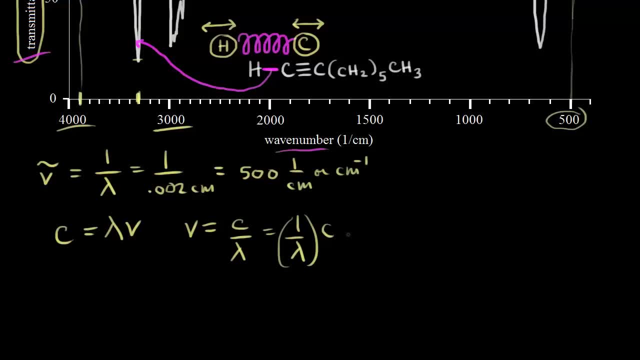 all right times the speed of light. One over lambda was our definition for wave number. So you could say that the frequency of light is equal to the wave number. all right times the speed of light. So let's go ahead and do that calculation here. 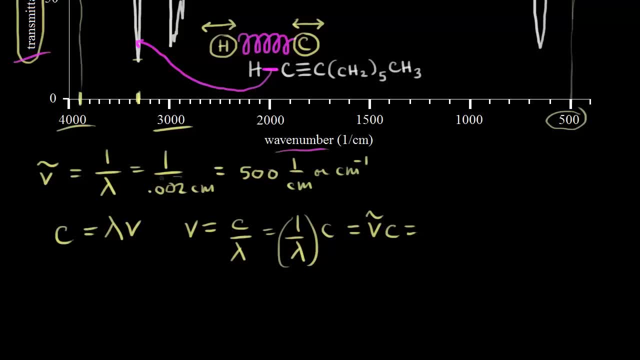 So for we talked about this as being a particular wavelength. all right, we found the wave number. Let's plug that wave number into here and let's see what we get. So the wave number was 500 units for one over centimeters. 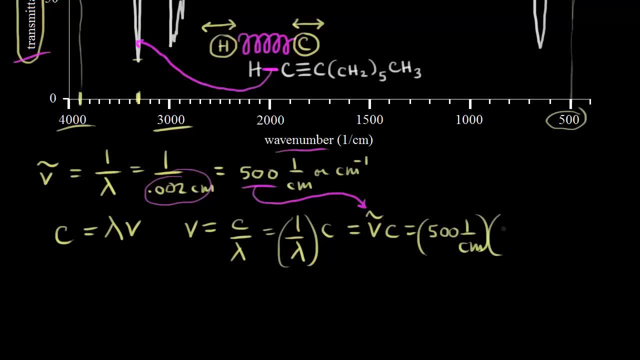 Multiply that by the speed of light. We need to have the speed of light in centimeters, so that's three times, approximately three times 10 to the 10th centimeters per second is the speed of light. Notice what happens to the units. 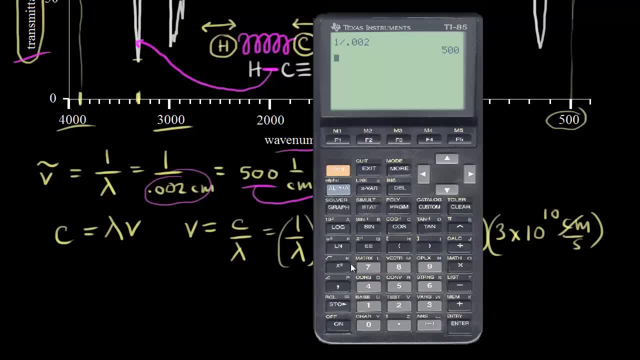 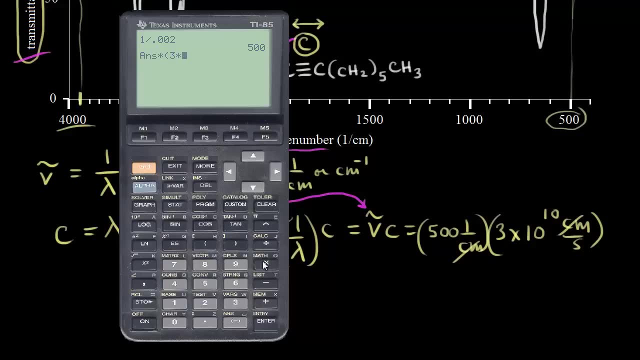 The centimeters cancel. and let's do the math. So let's get some more room down here, Let's go over here. So we take the wave number and we multiply that by the speed of light in centimeters. So three times 10 to the 10th. 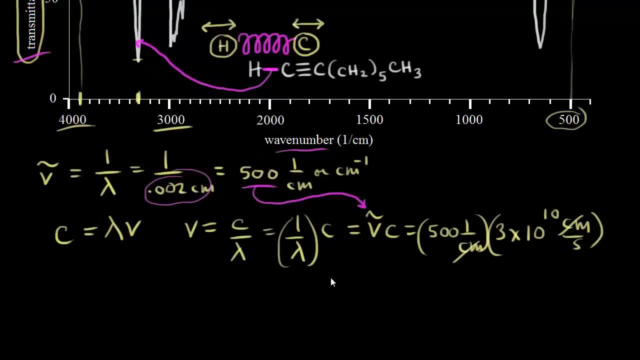 And we get 1.5 times 10 to the 13th. So the frequency: all right, the frequency would be 1.5 times 10 to the 13th. The units would be: this would be one over seconds. 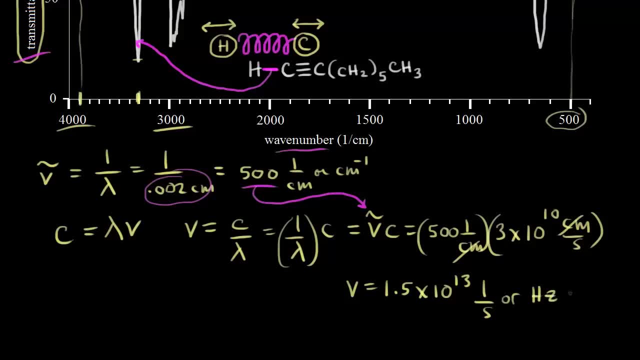 or you could say, or use hertz for that. So a wave number right corresponds to the wavelength and you can also get the frequency from that. So we have- let me just rewrite this really quickly- So frequency is equal to wave number. 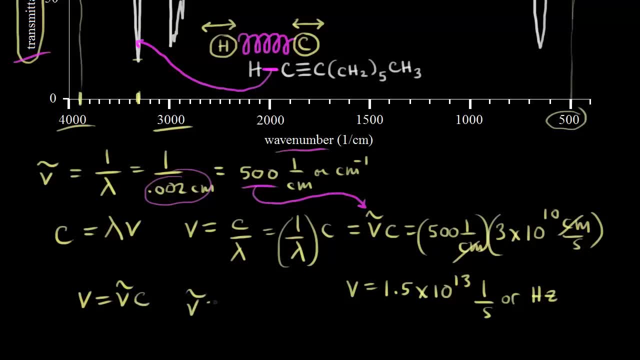 times the speed of light, And so wave number is equal to the frequency divided by the speed of light, And we'll use this in a later video. So we'll come back to this idea, But for right now the frequency of light is directly proportional to the wave number. 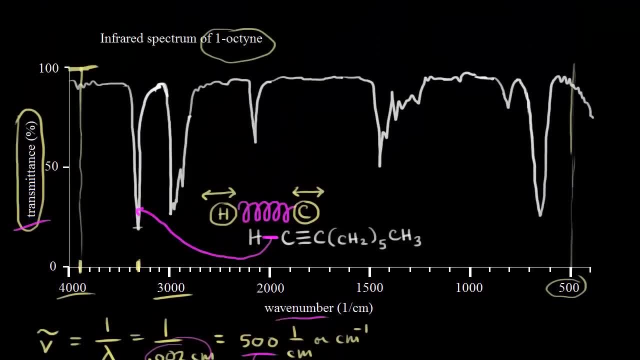 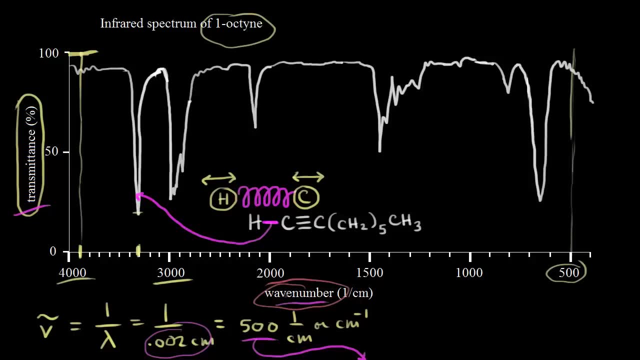 And so you could look at an infrared spectrum. Let me go back up here. You could look at an infrared spectrum. call this down here. you could call this a wave number. you could refer to it as a frequency. You could call it whatever you want. 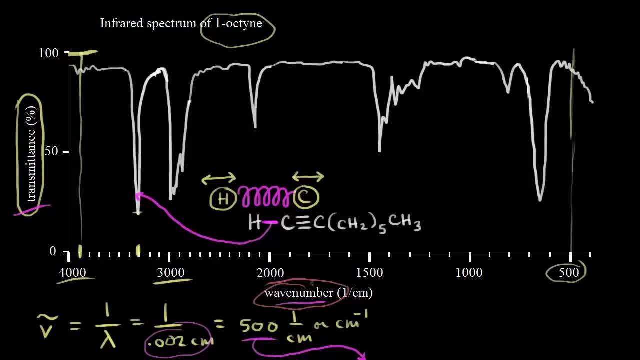 as long as you understand what's going on here, Let's look more in detail at this infrared spectrum And let's draw a line at approximately 1,500 wave numbers, right here And the left side, the left side of that line. 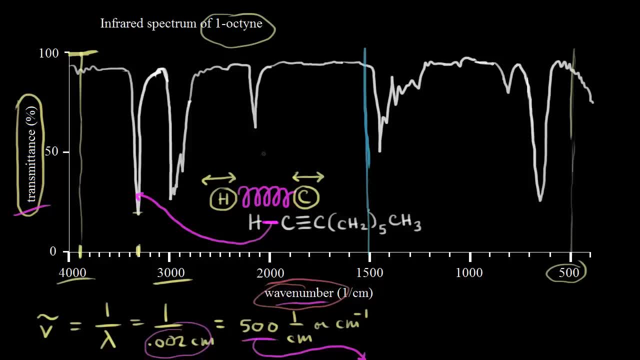 so we've divided our spectrum into two regions. The region on the left is called the diagnostic region, So this is called. this is called the diagnostic region of our spectrum, And it's because a signal in this region can be diagnostic for a certain functional group. 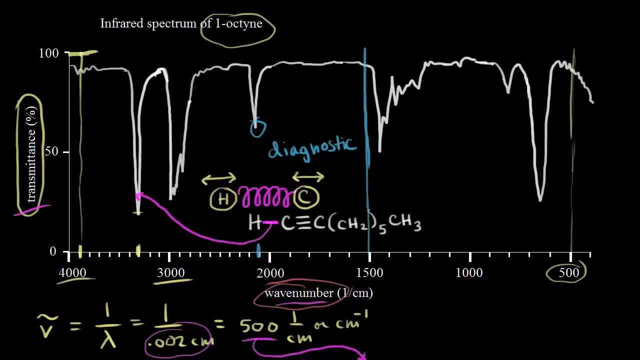 For example, this signal right here: if we go down here to the wave number, that signal's at approximately approximately 2,100,. right for this wave number here. And that's corresponding to the triple bond here. So this tells us a functional group right.